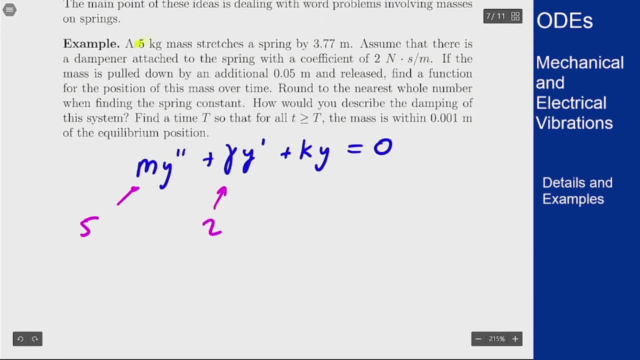 and the spring constant. here is two. All of these units in this problem work out so that this entire equation is here is in newtons, Right: kilograms times meters per second. squared newtons times meters per second. and then the spring constant times meters will get us the entire equation newtons. But the only thing we don't have yet is the spring. 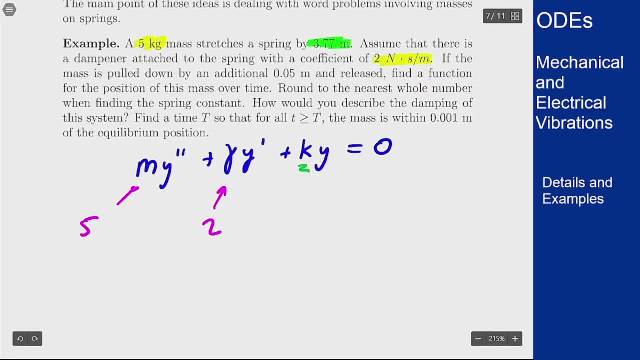 constant And that is actually hidden in this information here about how far this mass will pull down the spring. So when the spring itself is at equilibrium, it means that the mass pulling down or the force pulling down is the same as the force of the spring pulling it back up. 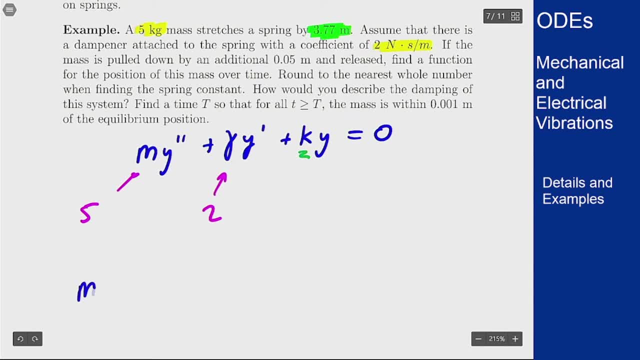 It means that we need to have that in that situation. mass times gravity- the force of gravity pulling down equals the spring constant times l, the length of the extension of the spring. We know everything in this equation except for k. We can solve this to get that 5 times 9.8 meters per second, squared for gravity. 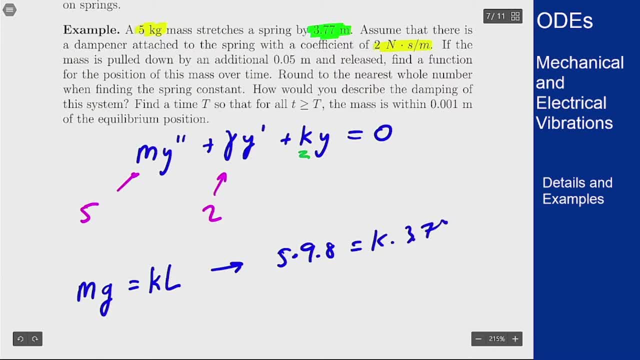 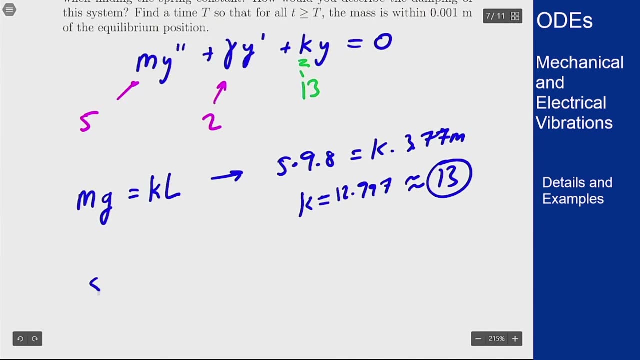 should equal k times 3.77 meters, And this comes out to about 12.997, or rounded comes out to 13.. So we'll use 13 here for this problem. So this means I'm left with the differential equation: 5 y double prime plus 2 y prime plus 13 y equals zero. But what about initial conditions? 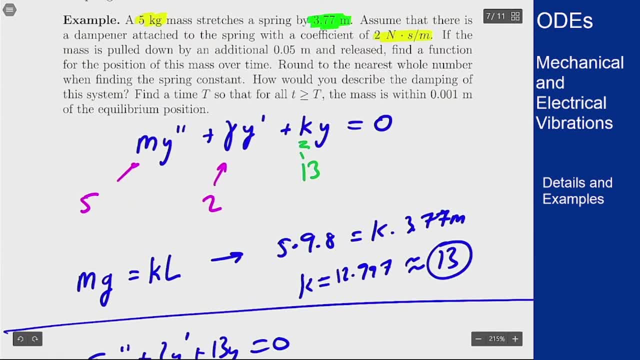 Well, in the problem statement I'm told that this mass will be pulled down by an additional 0.05 meters and then released. So the 0.05 meters is the initial displacement where it's pulled down that mark before it's released. So that tells me that y of zero equals 0.05.. And released means 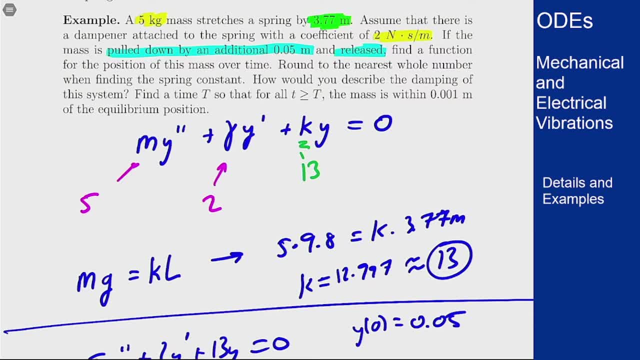 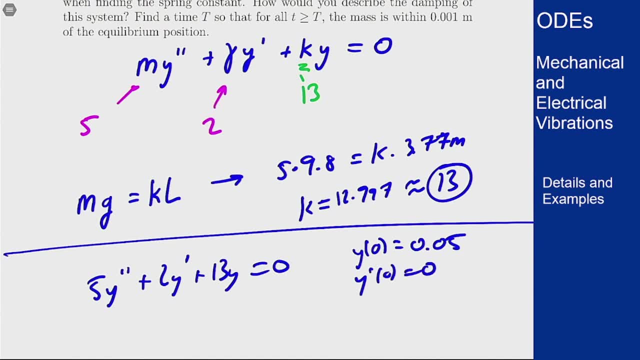 the initial velocity is zero because I have not put any extra velocity in it. when I've let it go, I've just sort of released it and let it bounce away. So y prime of zero is zero. Now we go try to solve this problem. So to do that we will start with the character equation of the system. 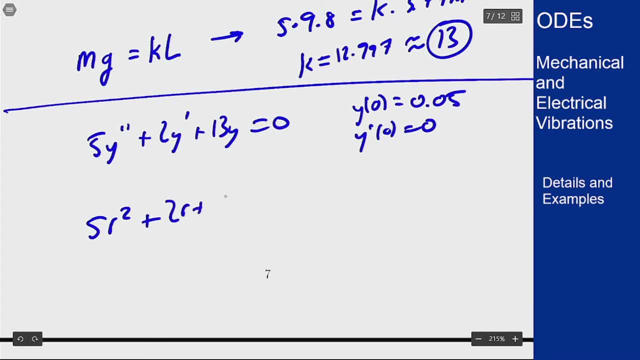 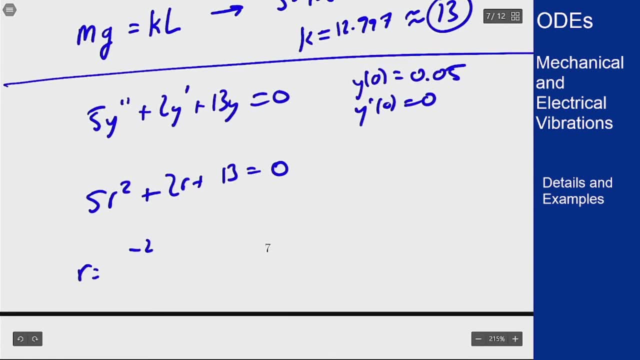 which is 5 r squared plus 2. r plus 13 equals zero. This doesn't seem to factor, So let's look at the quadratic formula for the roots We'll get. r is negative, 2 plus or minus the square root of b. 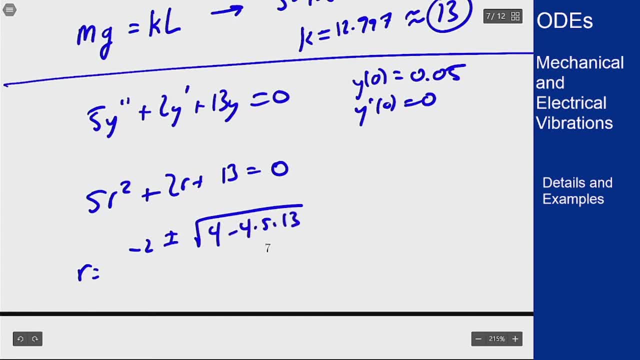 squared is 4 minus 4 a c over 10.. 2 times 5.. I'm going to get negative 2 plus or minus. square root of 4 times 5 is 20.. That's 260.. 4 minus 260.. 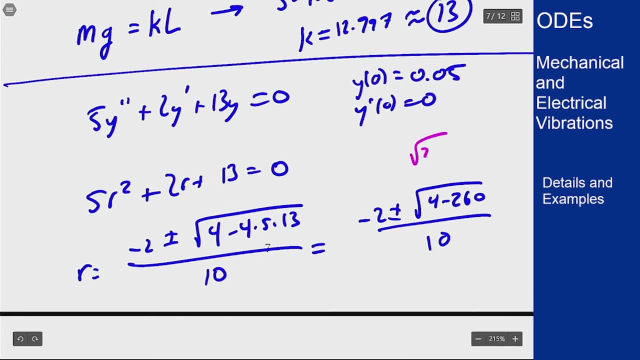 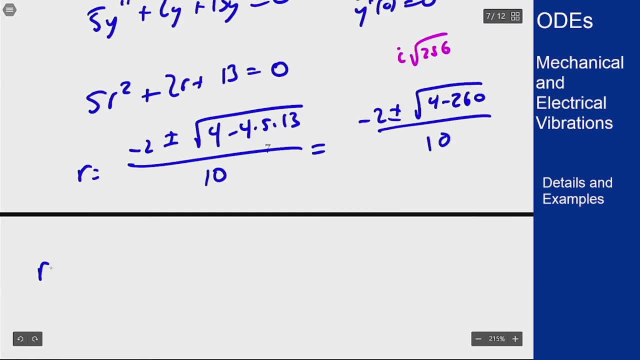 over 10.. This will be root 256, with a negative sign in front of it. So an i out front, And that's 16.. What I will see then is my roots are negative: 2 plus or minus 16 i over 10 or negative 1. fifth, 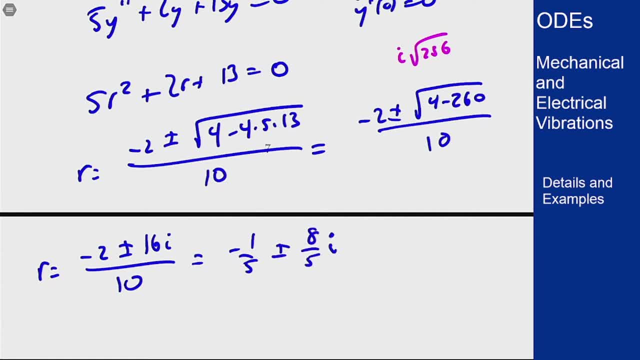 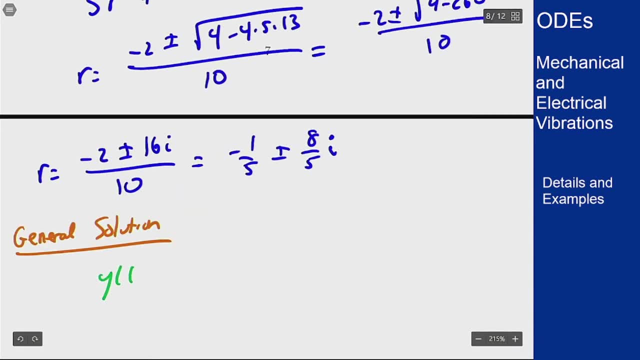 plus or minus 8 fifths i, So what that means. I can write my general solution to this equation as: y of t is c 1 e to the minus one fifth t. cosine of eight fifths t plus c 2 e to the minus one fifth t. 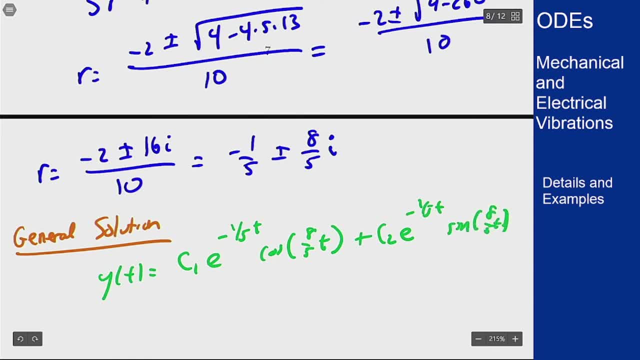 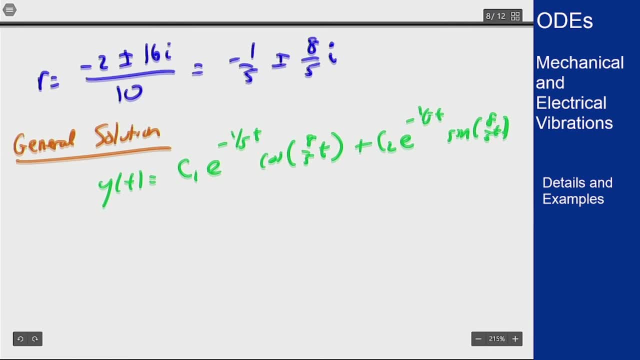 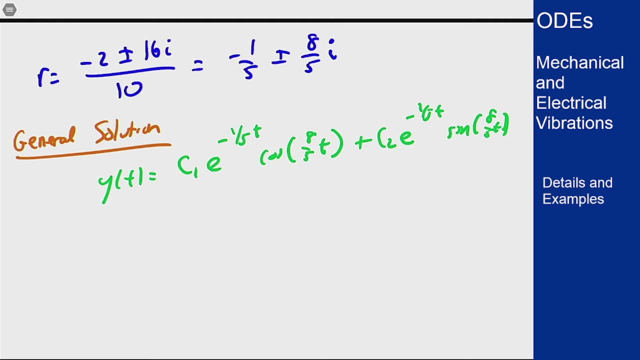 sine of eight fifths t. And now we can use this here to work with our initial conditions. Initial condition we have that we'll get something for y of zero, something for y prime at zero. I can work with y prime first and write out the formula here. This will be done by: 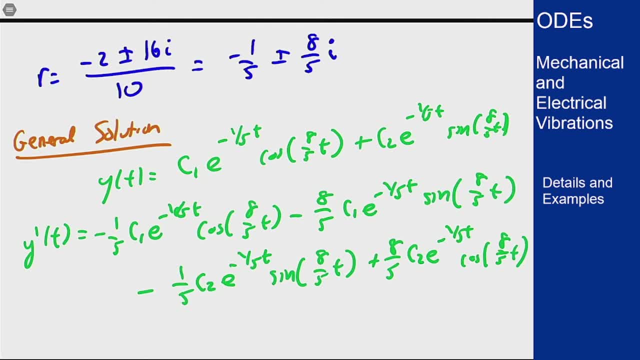 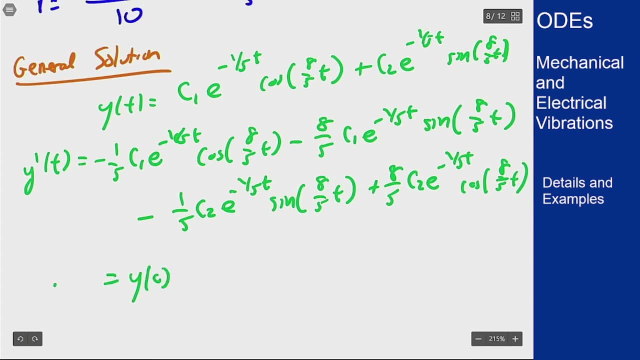 two applications of the product rule And when we plug in zero we can use that to find these constants. The y of zero we're assuming is 0.05.. And if I plug in zero for t up top here, I will see the sine term goes away, because that goes to zero. This goes to one. 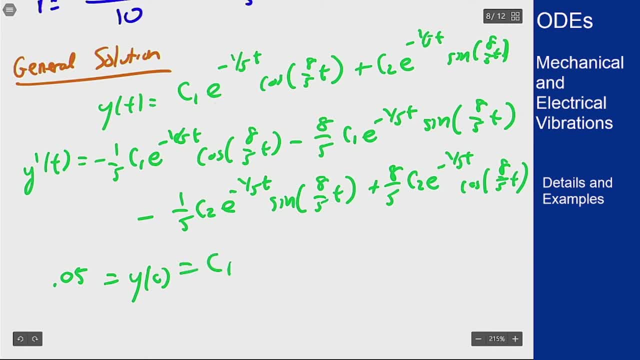 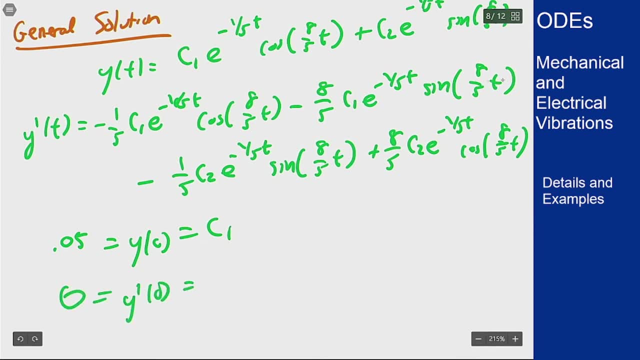 this goes to one. So I'm just left with c1 here, Fantastic. And then for y, prime of zero. I get this should be zero. And when I plug in zero here, both of the sine terms are going to vanish because they're both going to go to zero. I'll be left with a negative one. fifth, c1 plus an. 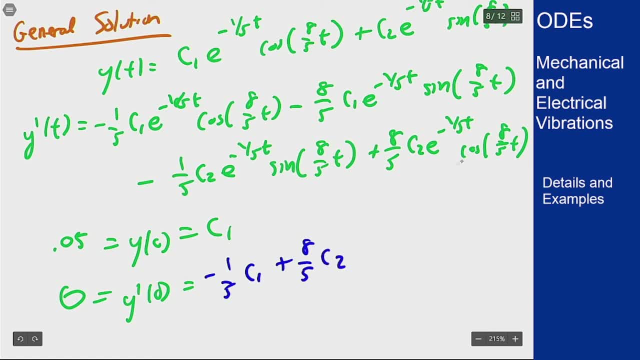 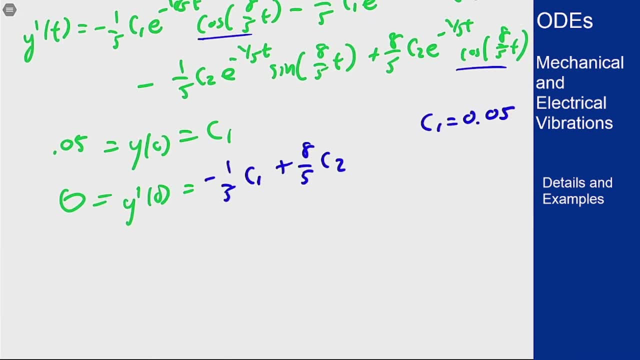 eight fifths c2 from the two cosine terms that are left. This tells me that c1 is 0.05 and c2- I can find- because if I add this term over I will get a 0.01 on this side- equals eight fifths c2.. So c2 is 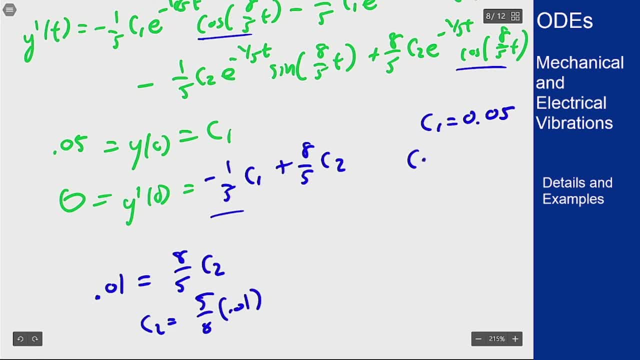 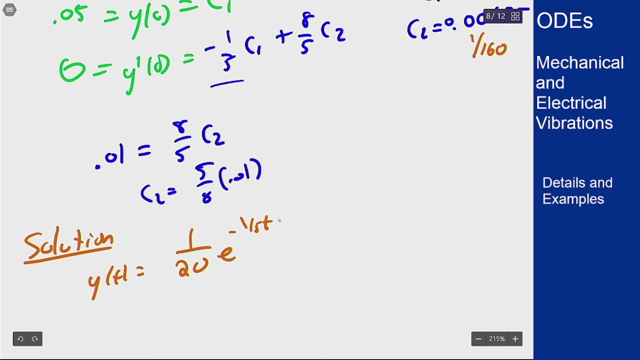 five eighths times 0.05.. 0.01 or 0.00625.. Or, if you want fraction forms, this will be a 1 over 20 and this will be 1 over 160.. So from that we get our solution. y of t is 1 over 20. e to the minus one fifth t. 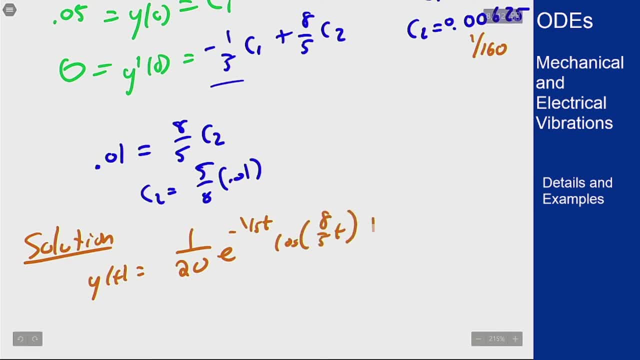 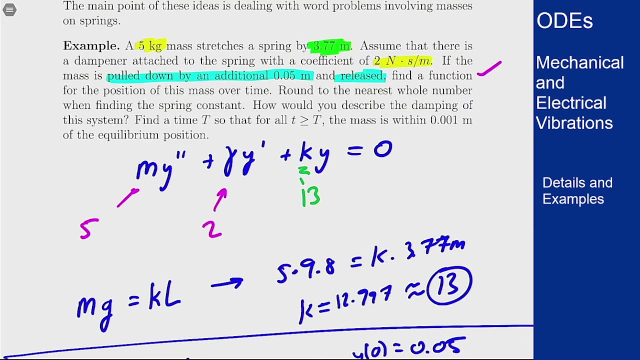 cosine of eight fifths t, plus one over 160 e to the minus one fifth t sine of eight fifths t. Let's go back and see what the problem actually asked us for. now We found a function, Good, Grounded, full number, Great The damping of the system. well, we're seeing. 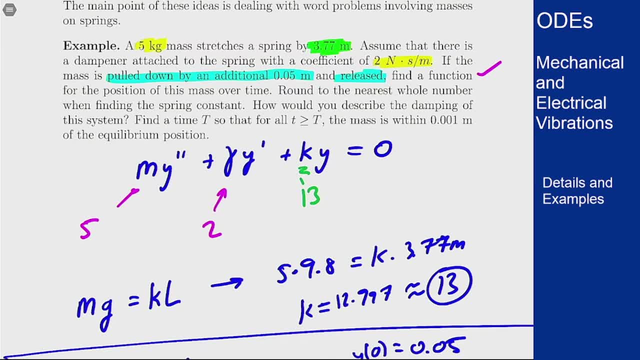 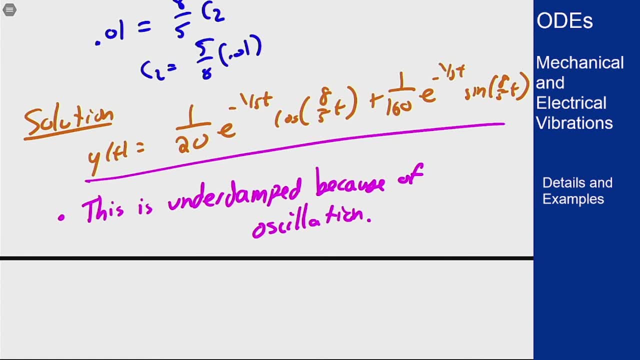 oscillations. So, because there's oscillation, this is an under damped system. And then, finally, we want to figure out when this object is within 0.001 of the original position. How can we do it? We first have to combine this into a single trig function to get the amplitude, to find the 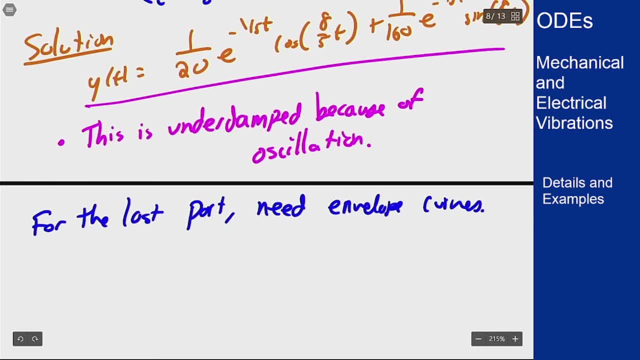 recurves for this And so for that, we know that we're going to get a amplitude That is square root of c12 plus c22.. So square root of 1 over 20 squared plus 1 over 360 squared, Which, since that is 1 over 20 and its 1 over eight, I will end up with a 1 over 20 root, 1 plus 1 over 64.. 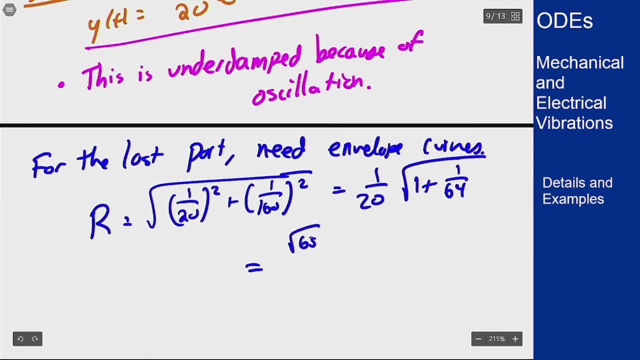 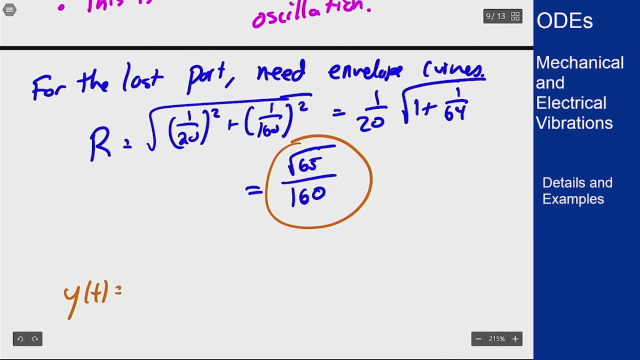 Which is simplified to a root 9 times 1 over 20.. 65 over 160.. This means I can rewrite my function here as y of t is root 65 over 160. e to the minus one-fifth t, cosine of eight-fifths t minus phi for some phi. Now I don't know what phi is and I could. 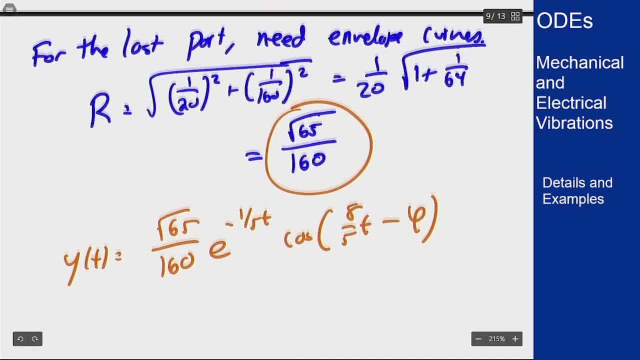 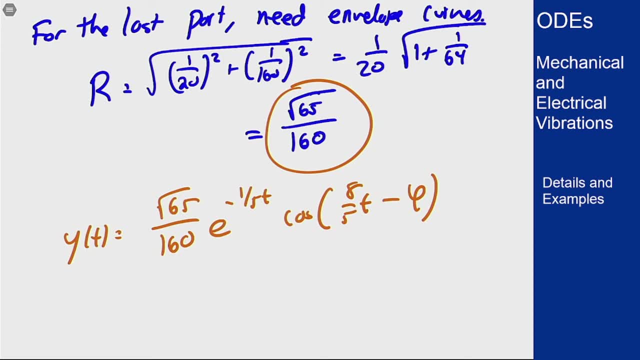 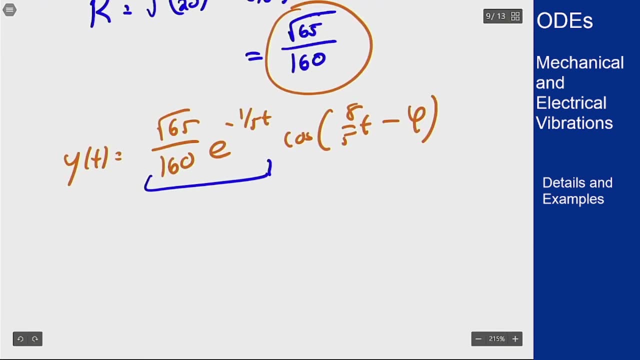 solve for it. but I don't need to answer this part of the problem. I want to know when. I know for sure this is within 0.001 of the equilibrium solution, which means I want to know when is this envelope curve, which is just this part, less than 0.001.. So to find this capital t, we want the root. 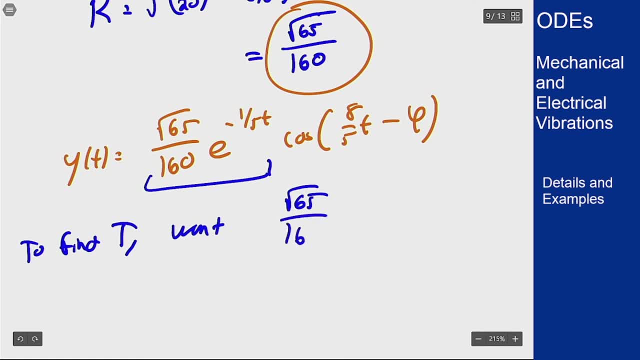 65 over 160 e to the minus one-fifth t, which is the envelope, curves here to be less than 0.001.. We can then solve for this. This means that you can solve for this. This means that you can solve for this. This means that.